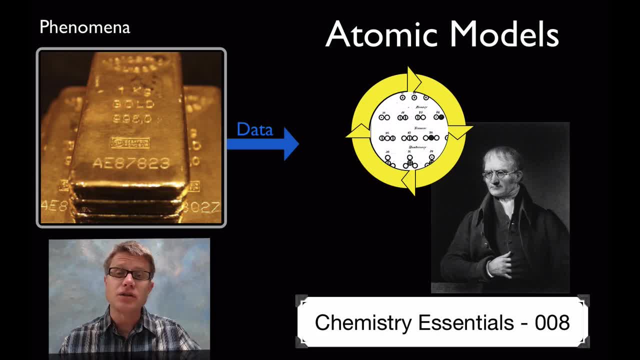 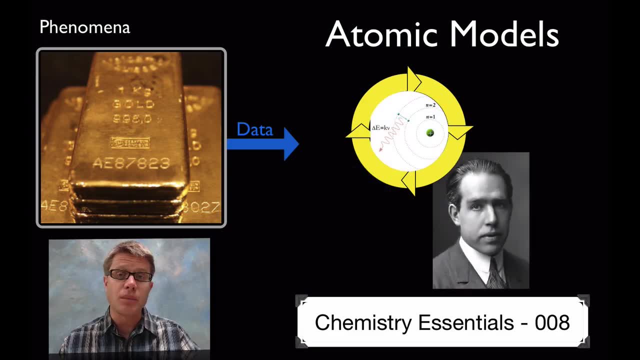 look like. So the Dalton model, that they were just these spheres that would connect, was a model. As we discovered the nucleus, we came up with Rutherford model, And then we use spectra to come up with a Bohr model, And then quantum given us more of this quantum. 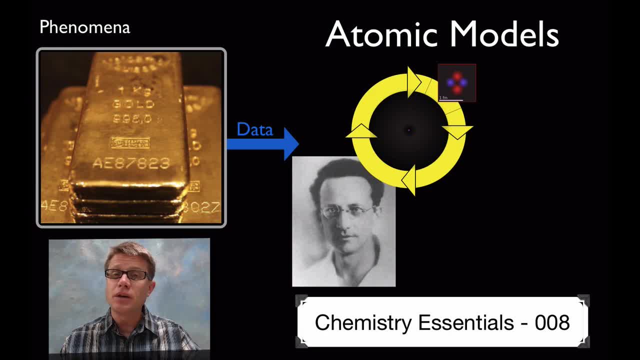 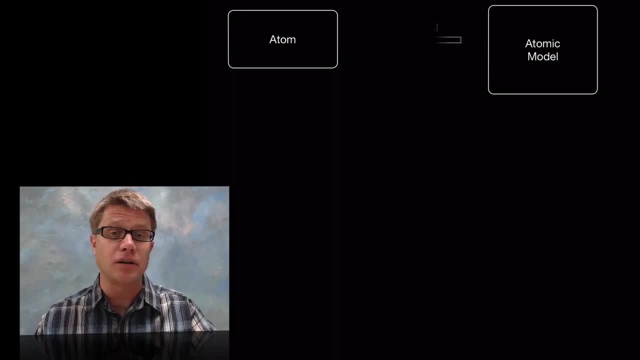 mechanical model developed by Erwin Schrödinger, And so we're improving this theoretical construct of what an atom is like. And so we've got an atom which is phenomena, and then we have an atomic model which is just a construct of what we think that looks like And what 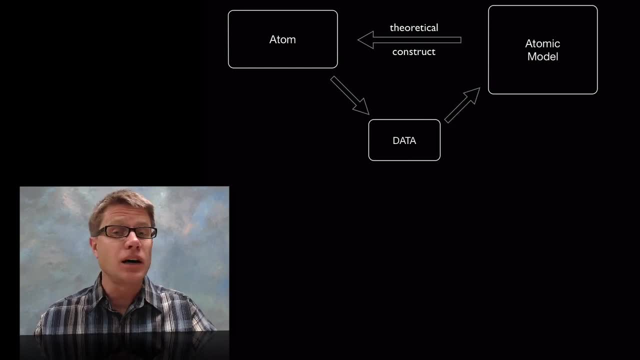 we're able to do is gather data from the phenomena, And as long as that fits our model, then everything is good. But what they were talking about there was a single atom which was going to look like an atom, Presumably an atom. It's a small atom that, likes, looks bigger when you put it inside an atom, if there areến. 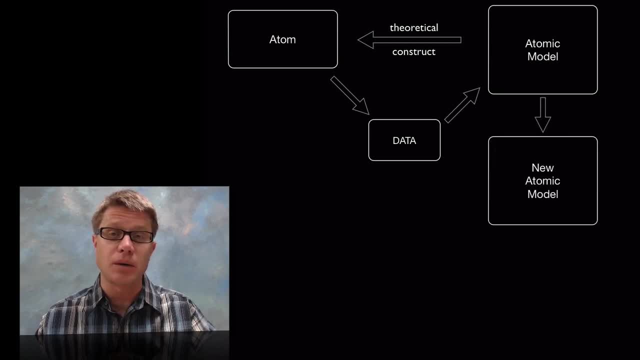 But once we start to conflict with that model, then we have to develop a new atomic model And we play that against the data. as long as everything fits, we use that model, But if it doesn't, then we develop a new atomic model. And that's really how science works. 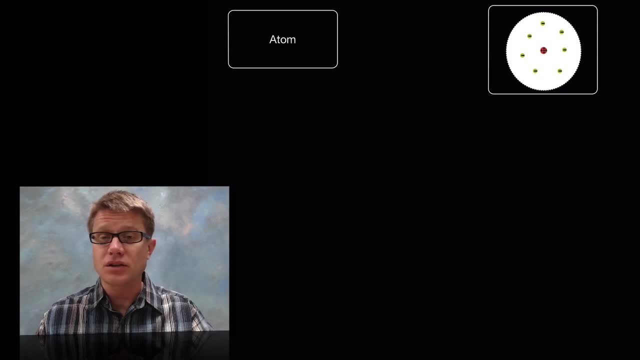 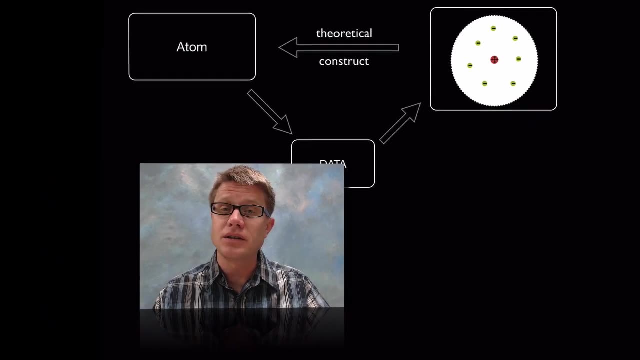 And so an example: if we're looking at the atom, the atom they used to once they discovered the nucleus and the electrons, this was our model, It's our theoretical construct of what an atom was like. But once the data didn't fit. once we got spectral data that said that 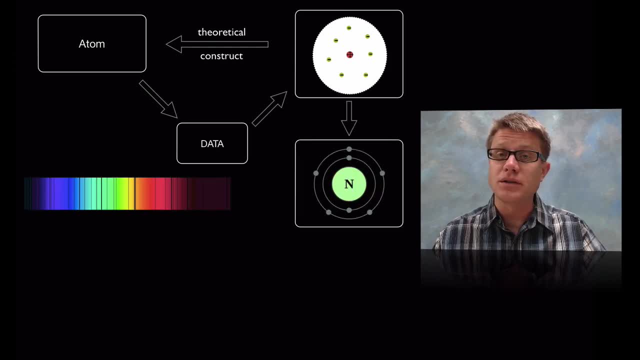 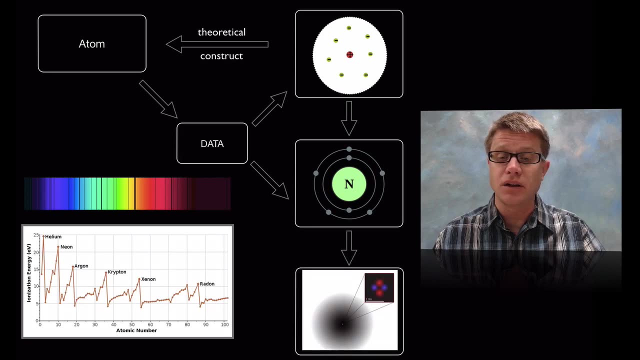 these electrons aren't just moving everywhere, that they're confined to orbits. then we came up with a Bohr model, And that worked until we started to look at ionization energy, learn more about quantum mechanics, and then we developed the model that we have today, And so, as long 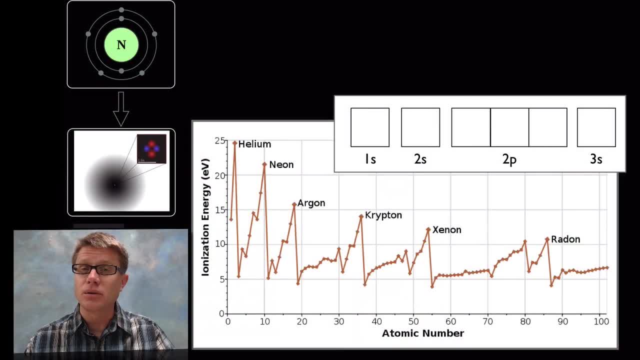 as that works, as long as it fits the data. that's the model that we're going to use, And so let's look at that one transition. How did we go from this Bohr model to more of a quantum mechanical model? Well, let's look at ionization, energy, Remember ionization. 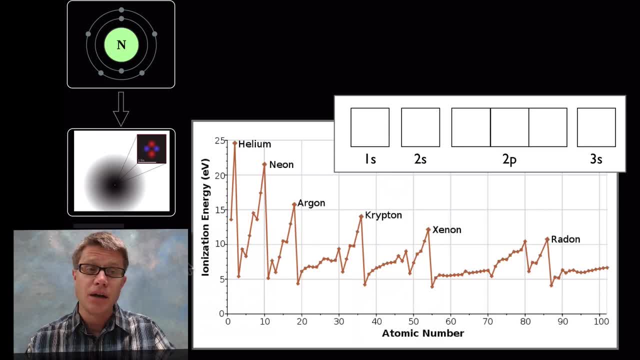 energy is the amount of energy it takes to pull an electron away. And so if this is the our model, you've got two electrons in the first shell, Then we'd go eight in the next shell And then we move out. like that, Ionization energy should be like this: Hydrogen to helium. 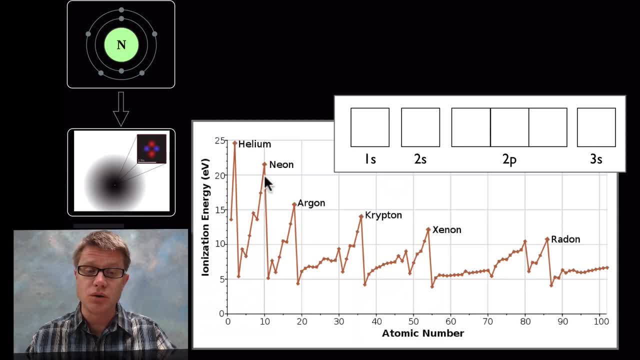 That works great. That would be the first subshell, But it should be really smooth as we move all the way from lithium to neon. But it simply isn't, And so we had to develop a new model, And that model consists of shells, and now subshells, And then those subshells.